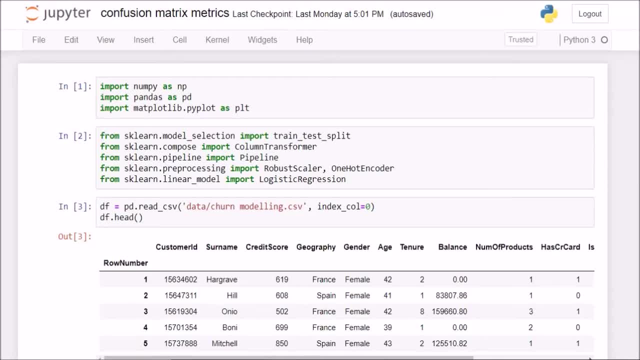 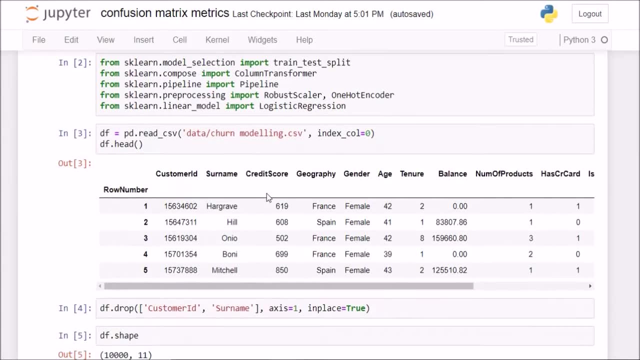 Namaste. in this session we will discuss how to code out the different confusion matrix metrics. okay, so i've imported all the necessary libraries that i'll be using and i and i'll be using the churn modeling data set, which has a set of people and the target variable is whether the customer 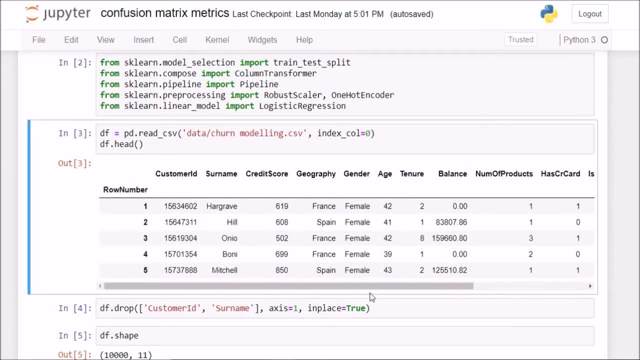 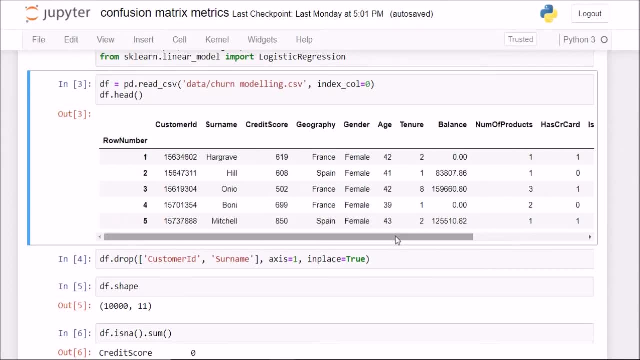 exited the bank or not. okay, so the customer has various features like gender, geography, age, tenure, balance. so, based upon these features, we have to predict whether the customer will leave the bank or not. now i don't think the customer id and surname have much importance when it comes to 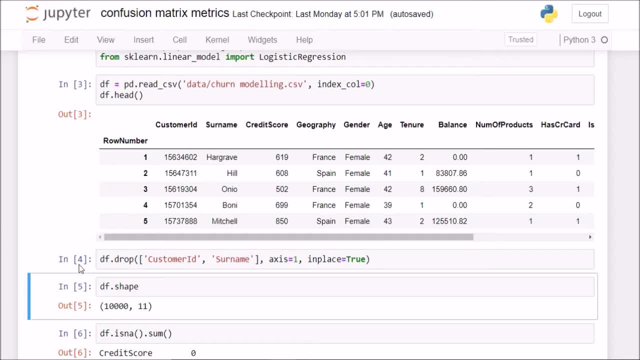 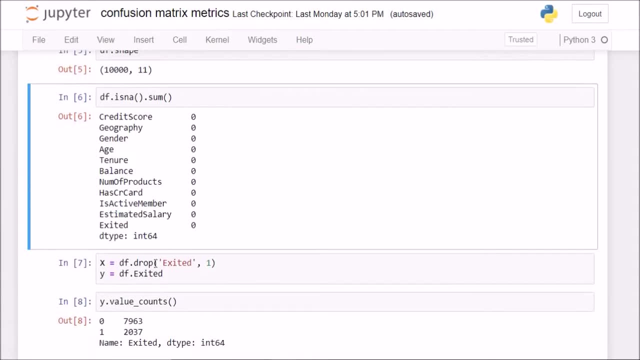 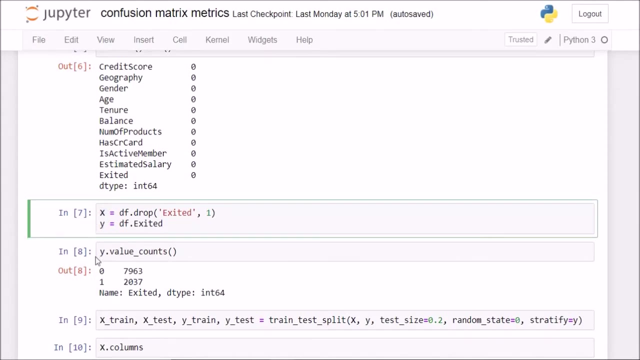 predictions. so i'll just be dropping them. and if i check my shape of my data set, i have 11 columns and 10 000 rows. okay, now, if i check, i do not have any missing values in the data. and now i'll segregate my data into feature vector x and target variable y. if i check my value counts, i have 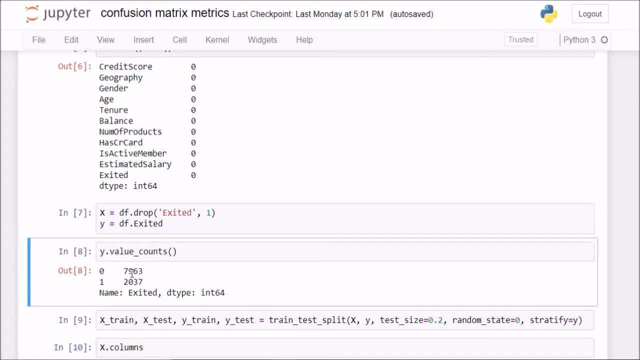 around eight thousand negative results, that is, eight thousand people did not leave the data set. and if i check the data counts, i have around eight thousand negative results. that is the bank and 2000 people left the bank. so there is a kind of class imbalance. so we need 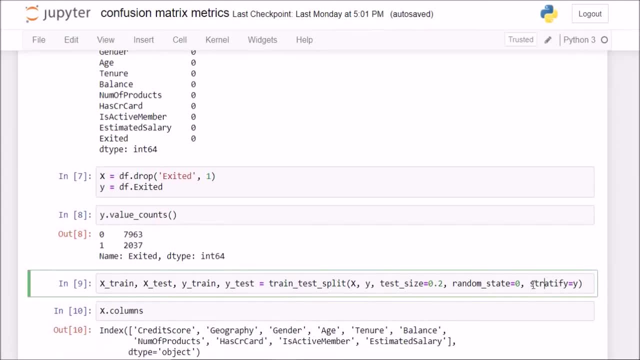 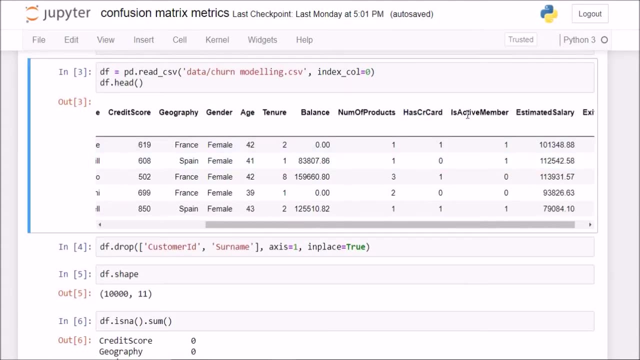 to keep this in mind when we are doing the train test split that we need to specify. the stratify is equal to y parameter. now, if i check my data, i have two columns here. has credit card and is active member. so both of these, although these are numerical features, 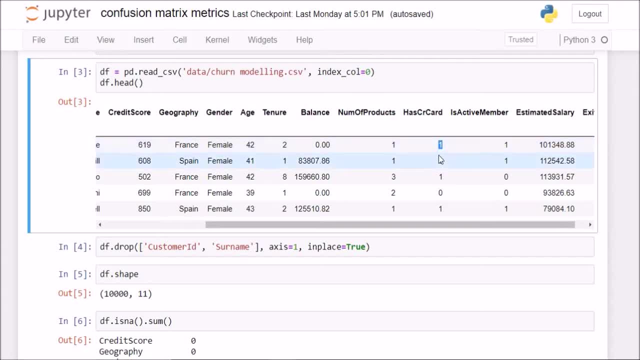 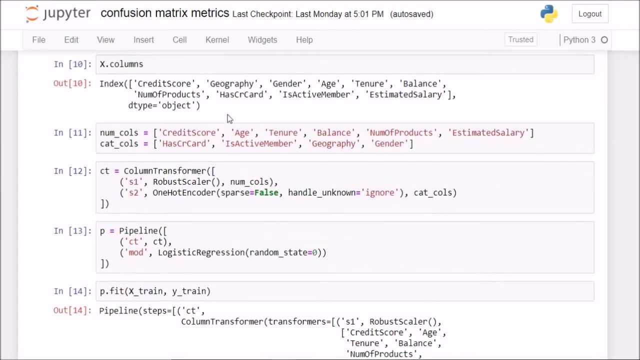 they are actually categorical features. one means the customer has credit card and zero means the customer does not have one and is active member. one means yes and zero means no. okay, so these are categorical features and hence i'll be including them in my cat calls list. now i'll simply robust scale my all my numerical columns and one hot encode. 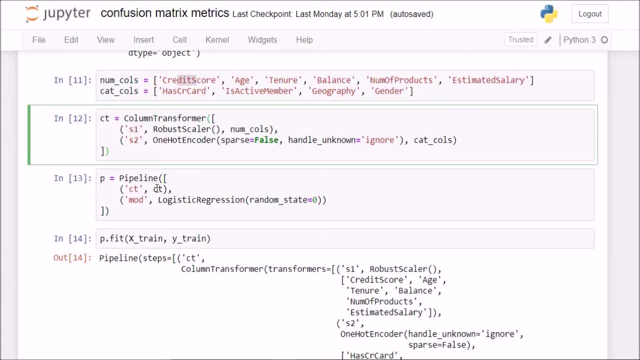 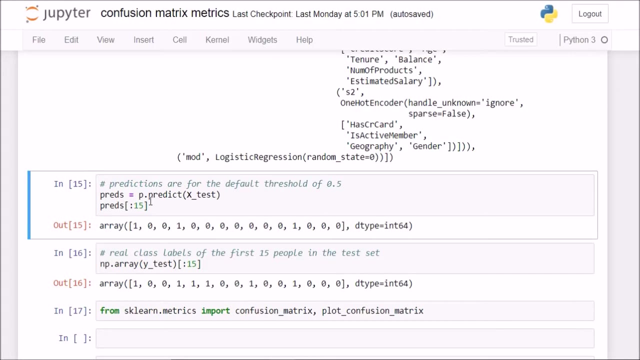 my categorical columns, and now i'll just pass them in my pipeline here, this ct object at the end of it, and, and as my last step of my pipeline, i'll be fitting a logistic regression classifier. okay, so, after fitting my classifier, it is time to do the predictions and these: 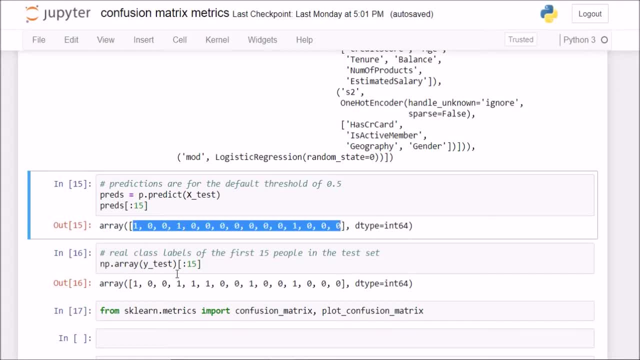 are my predicted values okay for the first 15 people in the data and if i check my real 15 values of the first 15 people, i see that the first person was directly classified to leave the bank and this person, this fifth person who did not, who was predicted to not leave, 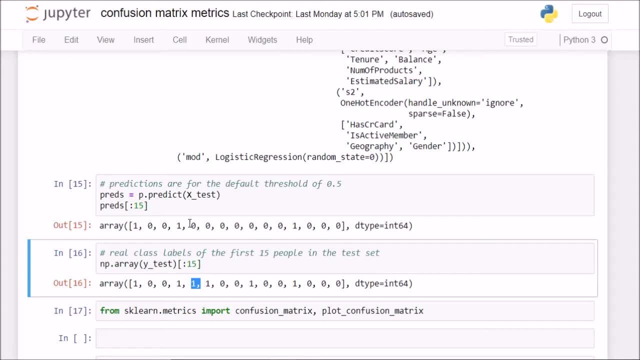 the bank, but in reality the person did leave the bank. so it was a case of false negative, and this is what we'll be trying to picture in the confusion matrix at how many two positive, true, negative, false positives and false negatives were there, and for that we got the part where we classified it and when we gl: Earth度-sat to n- 아니에요. 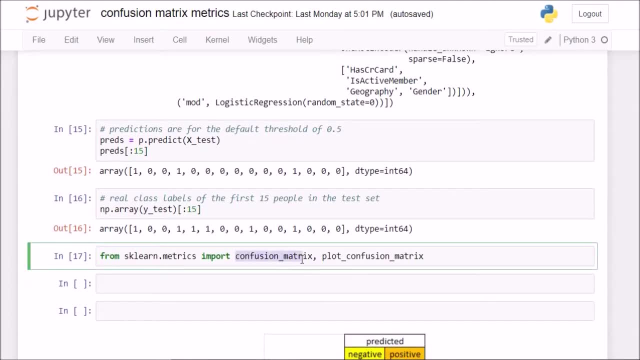 many true positives, negative false positives and false negatives where there, and for that and for that we will be using two carbons in unit plate, second part, and 40 mq n1 investigating. i have imported the confusion matrix function or the class from the sklearnmetrics module. 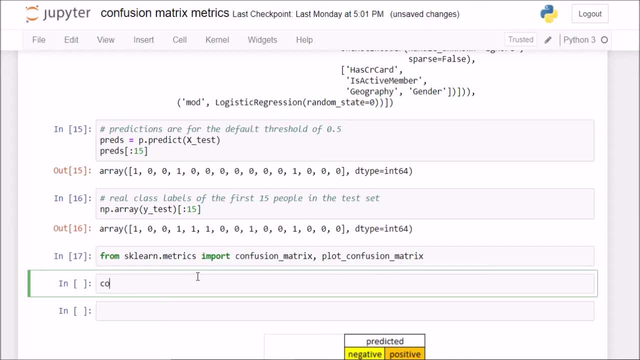 okay. so, first off, what i'll do is i'll say confusion matrix and if i check the documentation, it is asking me for for y true and y pred. so my y true, these are my y test values, my y pred, what are my y preds? well, these are my preds, which i've just calculated here. okay, so now, if i press, 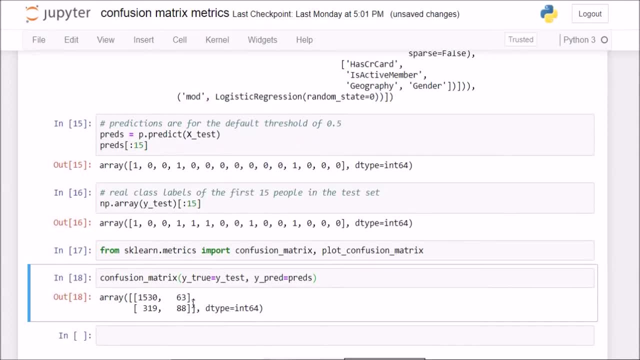 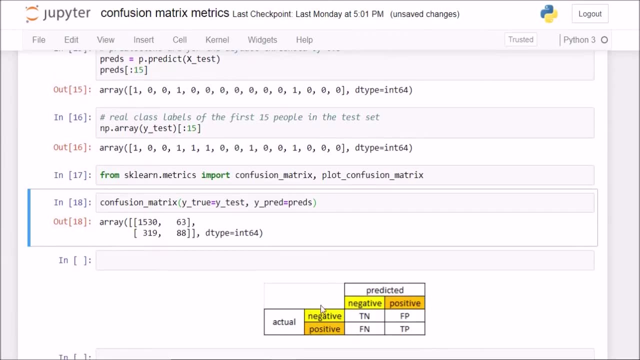 ctrl enter. i'll get this kind of a confusion matrix. now you must be wondering which one is the actual class, which one is the predicted class and which one is the negative and which one is the positive. well, by default, scikit-learn uses this kind of implementation where the actual is on. 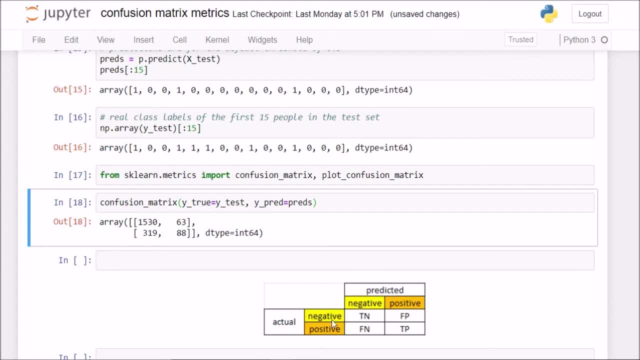 the row level and the columns are the predicted level, and the negative and positive are assigned in such a way that if i check my pclasses underscore, i'll get 0 and 1 right. so 0 is my negative class and 1 is my positive class, and hence 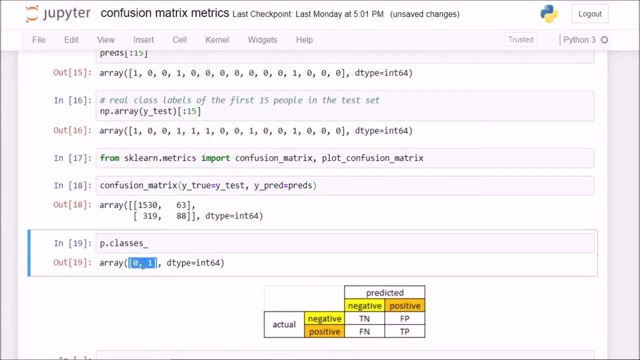 0 is my negative class and 1 is my positive class, and hence scikit-learn has sorted this classes array and hence i have negative first and positive second. so basically this 1530 is my true negatives, 63 are my false positives, 319 are my false. 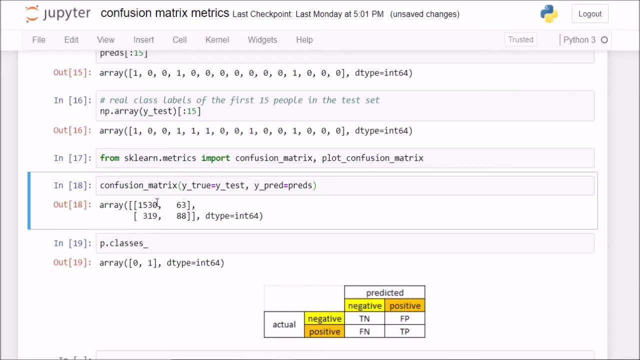 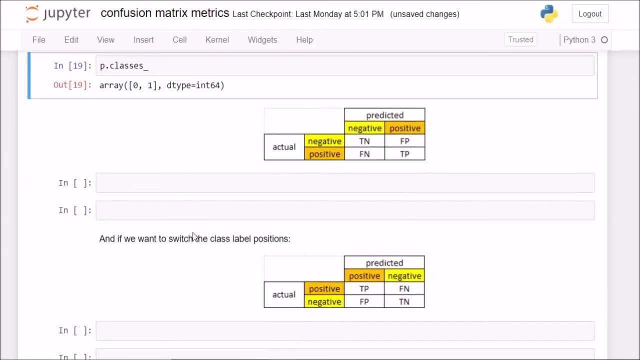 negatives and 88 are my true positives. so this is how we decode our confusion matrix. so now, what if you want the positive to be up and negative to be down, something like this? okay, so it is quite simple to do that. so what we'll do is i'll simply say the confusion matrix. 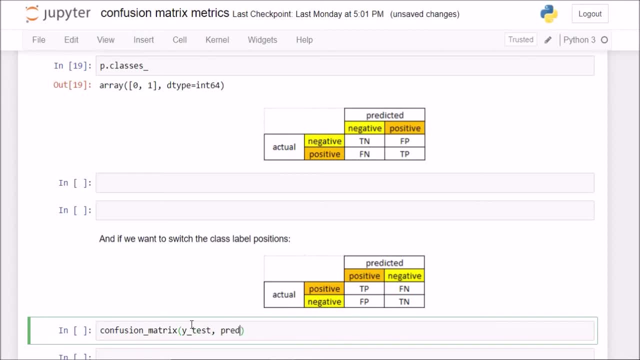 and again, i'll pass in my y test and my preds these two arrays, and next i'll also pass in an argument called labels, and this will be equal to 1 comma 0. okay, so i know that scikit-learn has chosen 0 and 1 to be the order, but i want the order to be 1 and 0. that is, positive and negative class. 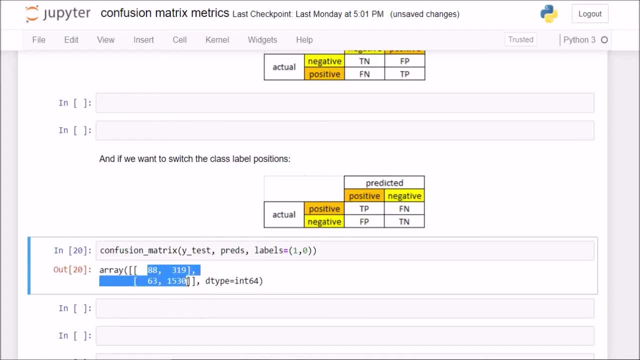 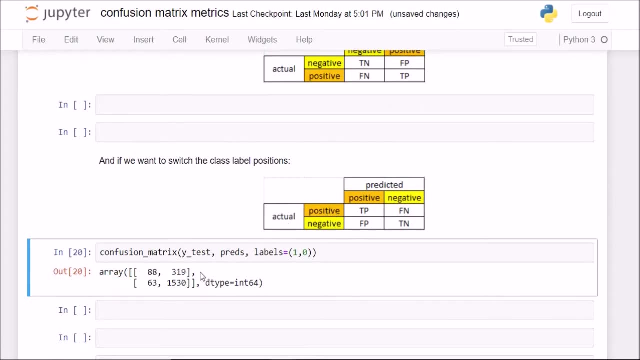 and when i press ctrl enter, i get this confusion matrix, which is the same as last one if i check. but the only difference is now my positive is up and negative is now. we need a way to extract information from these four values. what i'll do is i'll just. 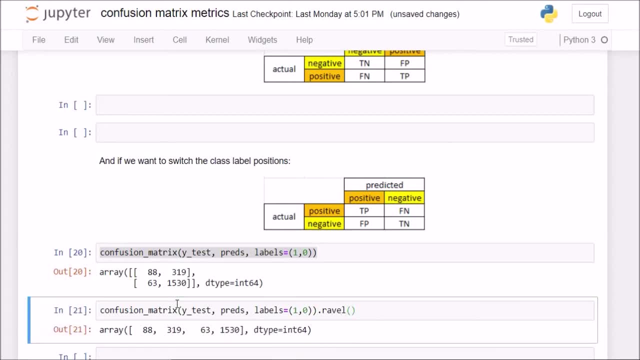 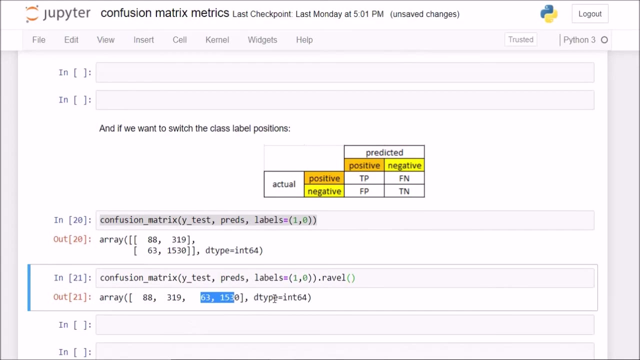 copy this here and now. i will say dot ravel when i say dot railway. it will simply just put one row beside the other. so this 83 and 319, these are, this is my first row, and 63 and 153 was my second row. so these are just put one beside the other. okay, so these are, just converted it into. 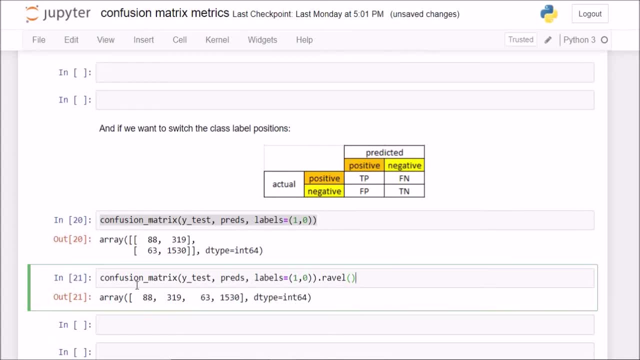 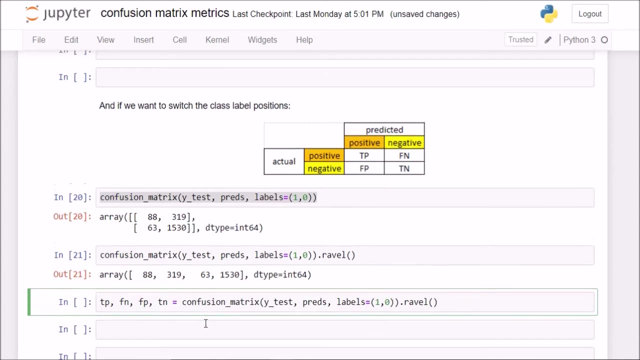 do a 1d array and now i know that 88 is my true positives, right? so what i'll just simply do here is: i'll say: true positive is my first one. second, i know that 319 are my false negatives. so i'll say false negatives, then my false positives and then my true negatives. so these are my four values. 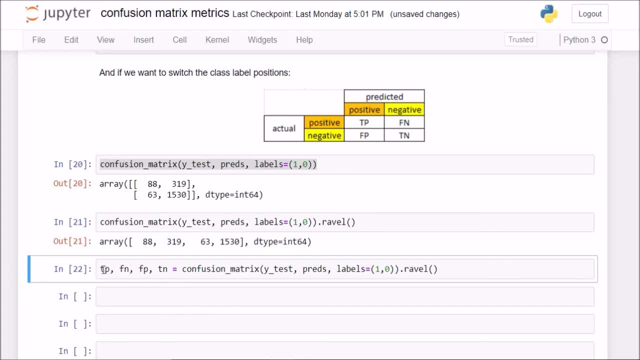 in this order. now i have successfully extracted information from this confusion matrix and now i can calculate, for example, my precision. my precision will be equal to true positives upon true positives, plus false positives. if i check out my precision value, it is 58.27 percent. now. 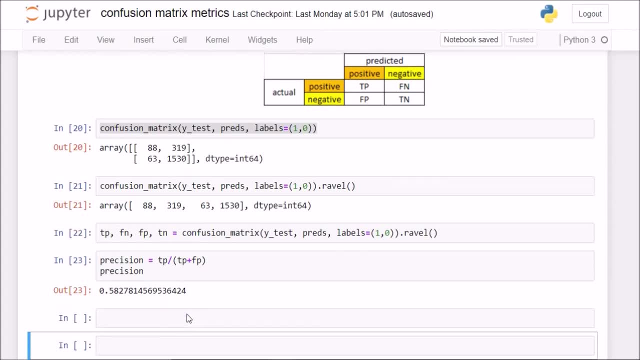 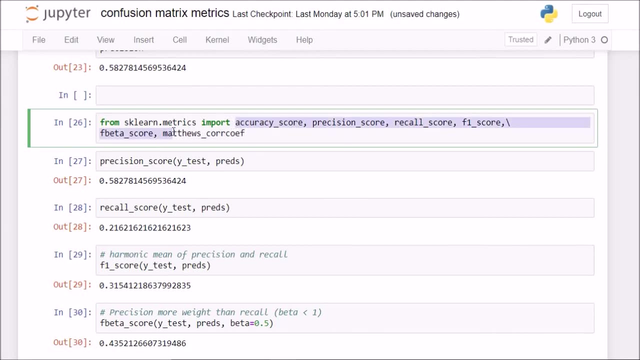 there must be an easy way to calculate all of these things right. so scikit-learn has done that thing for us. it has given us these functions of accuracy, precision, recall, f1 score, f beta score and matthew's correlation coefficient scores, and others as well, which are available in: 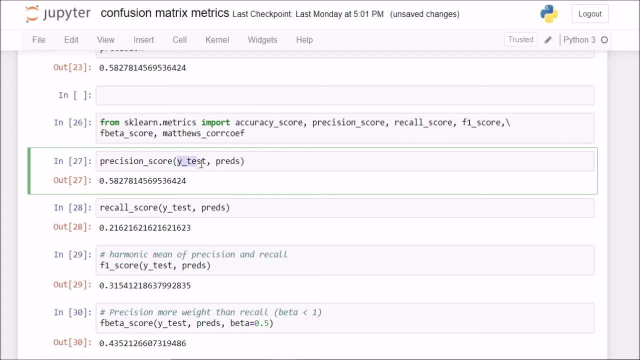 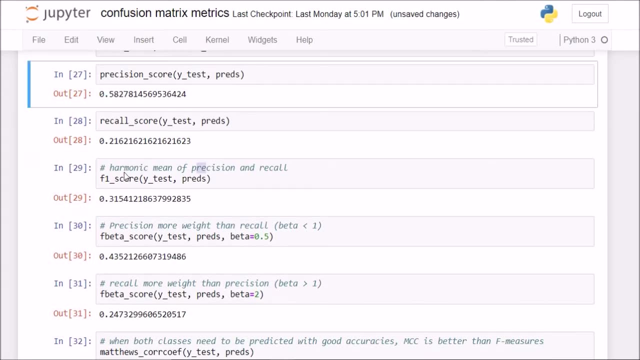 scikit-learncom dot matrix and we just need to pass in the y test and the predicted values and this will calculate the values for us. okay, we find that my precision was 0.6. my recall was very low at 0.21 or 21 percent. f1 score is 31 percent now for my f beta score. 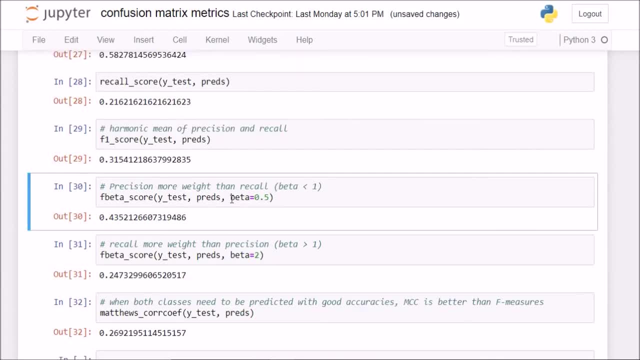 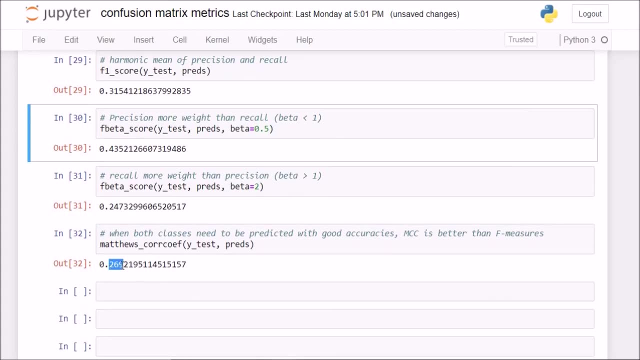 i can provide an argument called beta, and the choice of beta depends upon a business use case. and next, we can also calculate the matthew's correlation coefficient, which is 26 percent in this case. and we can also calculate the matthew's correlation coefficient, which is